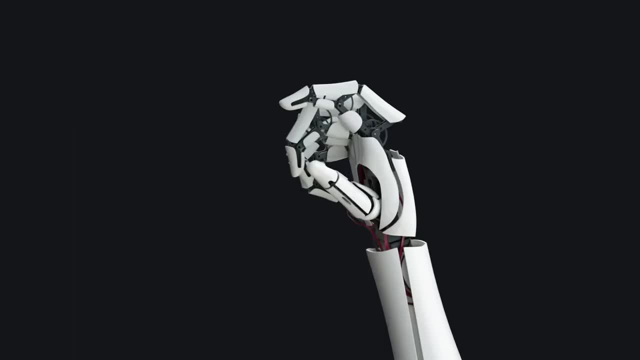 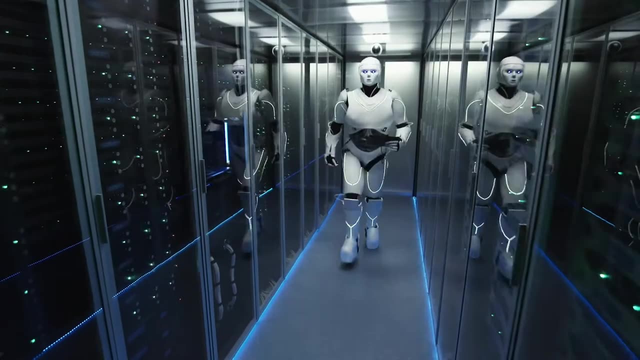 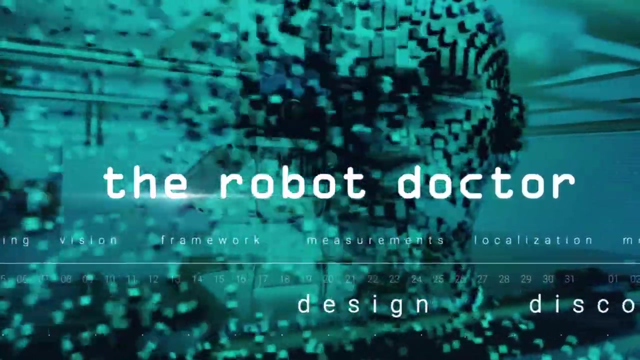 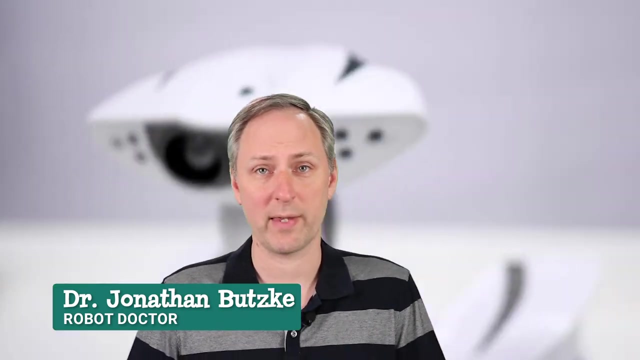 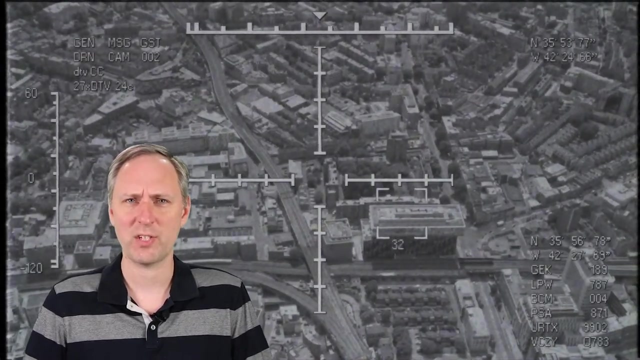 Hello, my name is Dr Jonathan Butzke. I'm not a medical doctor. Instead, I'm the robot doctor. Robots need to be able to sense their surroundings, and a common way of them doing that is with eyes made out of cameras. Cameras are handy sensors for a robot, because it allows them to see the 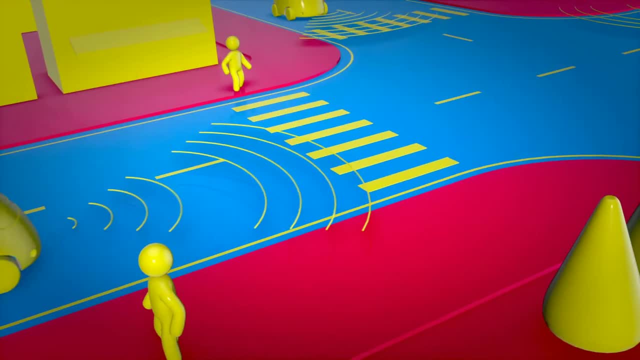 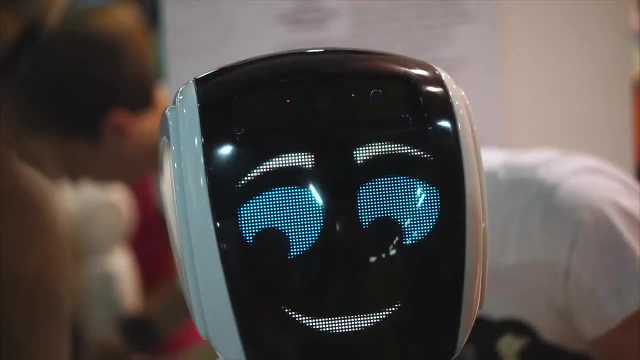 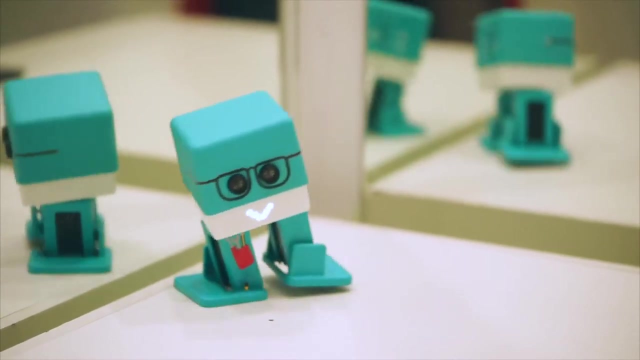 same sorts of things that people see. For example, a self-driving car can use cameras to see stop signs and lane lines, A robot receptionist can see and identify people and a small mobile robot can see obstacles and avoid them. In this lesson, we'll talk about vision- how robots see things. 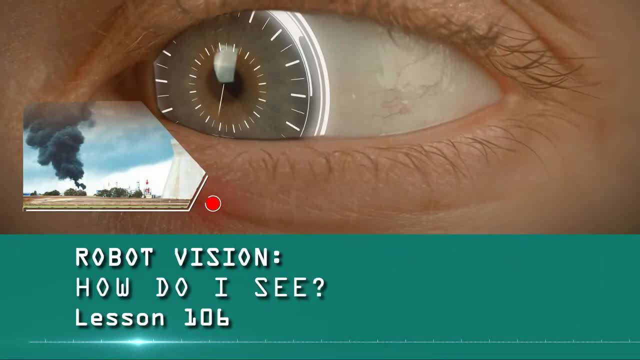 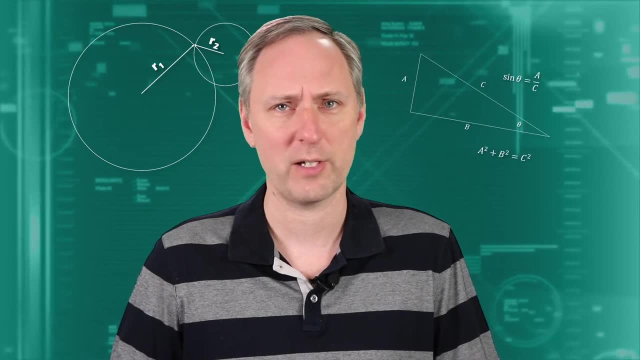 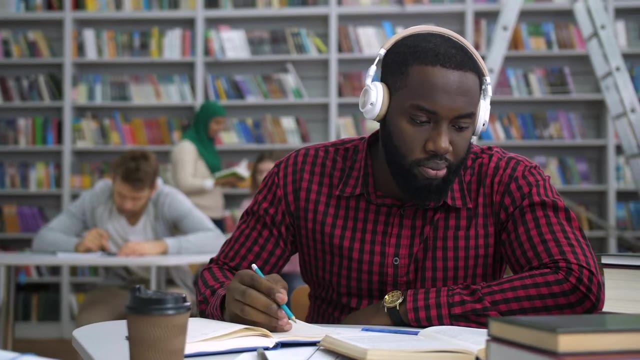 and how they can extract information such as distance from a set of images. And we'll do all of this using the math you already know: geometry, trigonometry, algebra and a few concepts from physics. Today, we'll explore points in three dimensions, so be ready with your pencil as we 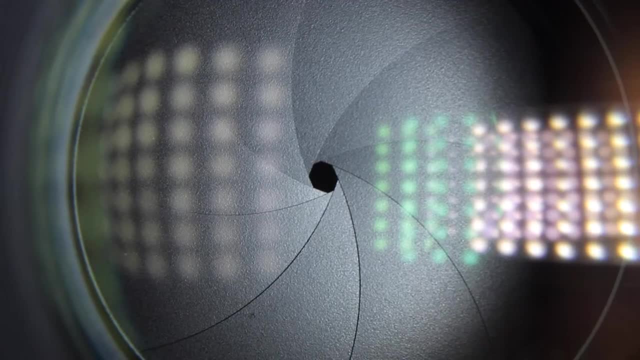 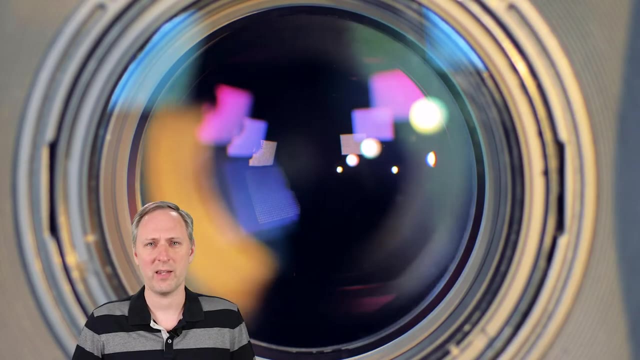 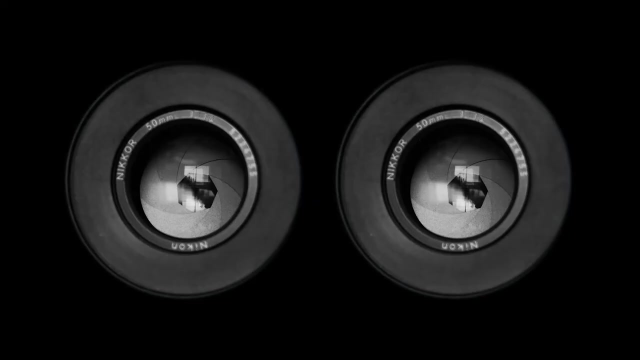 get started. Cameras are a very popular option for robots because of their similarity to human eyes, their relatively low cost and the abundance of algorithms. One such algorithm is the stereo vision algorithm. This algorithm allows the robot, using two cameras, to calculate the distance to nearby objects. For example, our robot can use 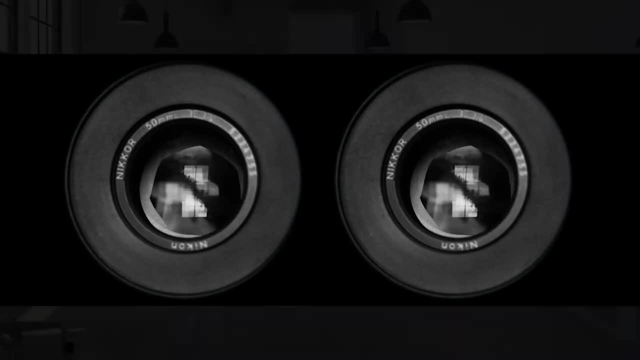 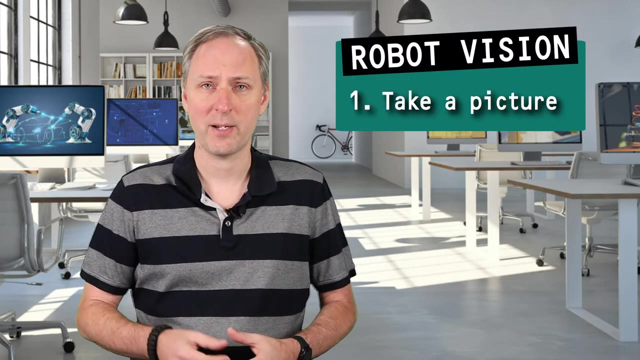 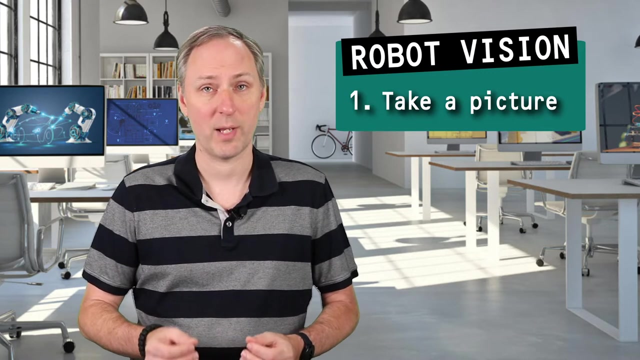 stereo imagery to avoid running into a tree as it drives around. To explore this aspect of robot vision, we will follow three steps. Step one: take a picture. This step produces an image, a two-dimensional representation of the real world. Step two: process the image. Find interesting. 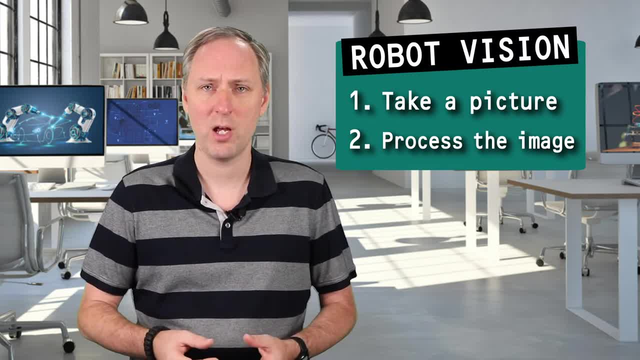 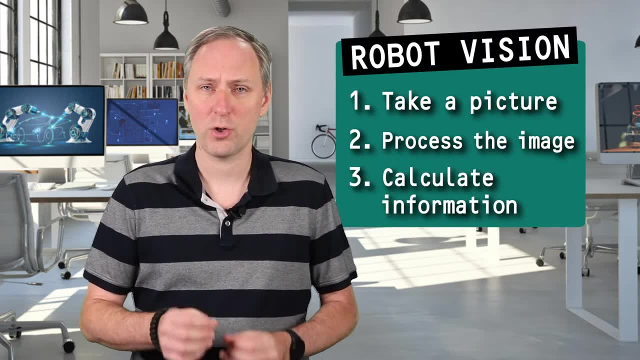 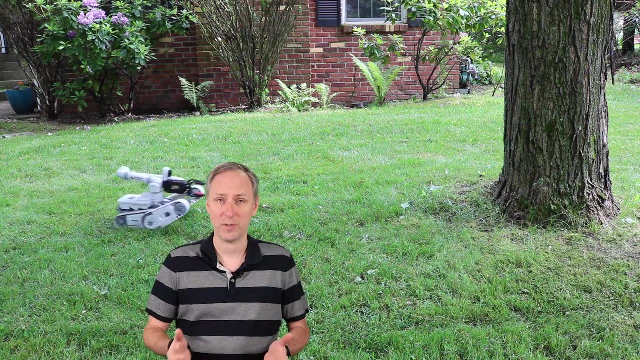 points such as corners and edges of objects in the image. We'll call these interesting points features. Step three: calculate information. Use the features to extract information about the scene, such as where objects are or the distance to particular features or which objects 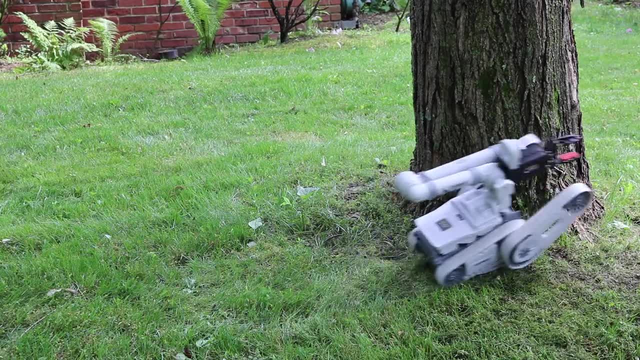 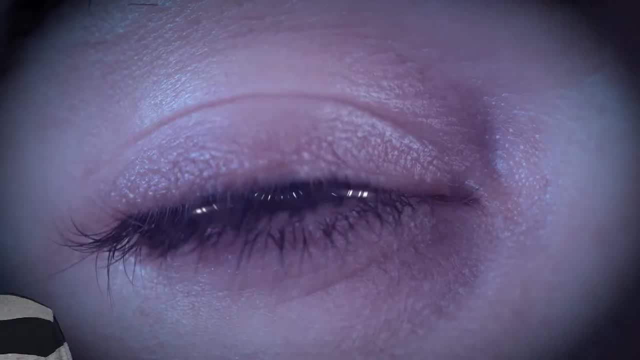 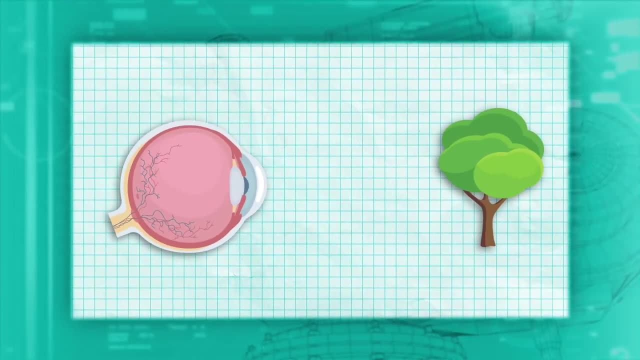 are in view. Hi Robot, You see that tree. To better understand robot vision, let's compare robot cameras to your eyes In order to see an object in front of you. light from a light source bounces off. the object goes. 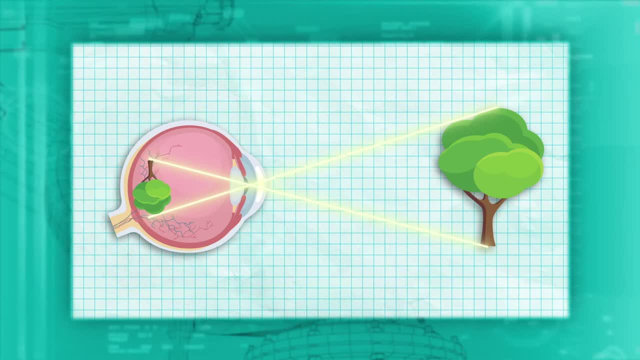 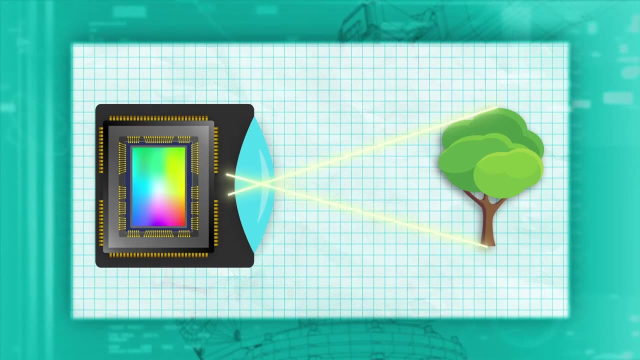 through the lens in your eye and forms an image on your retina. A robot's camera eye works the same way. Light bounces off an object, goes through the camera eye and bounces off the original object, which is the lens. I'm answering this question correctly. 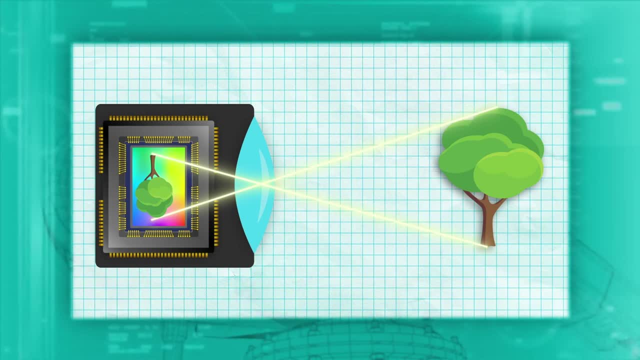 Let me go back to the room and go to my apartment next to that object. Hey Robot, You got to see that tree. To better understand robot vision, let's compare robot cameras to camera's lens and forms an image on the sensor. The camera sensor itself is fairly small, Usually. 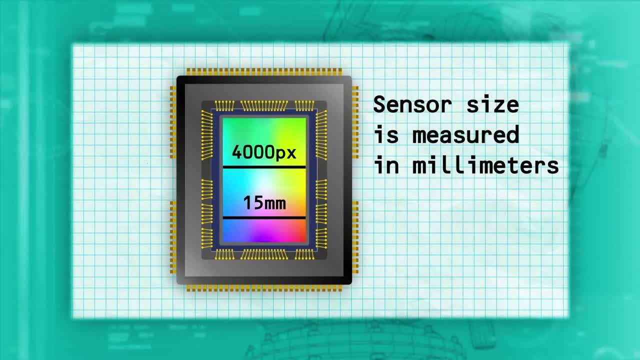 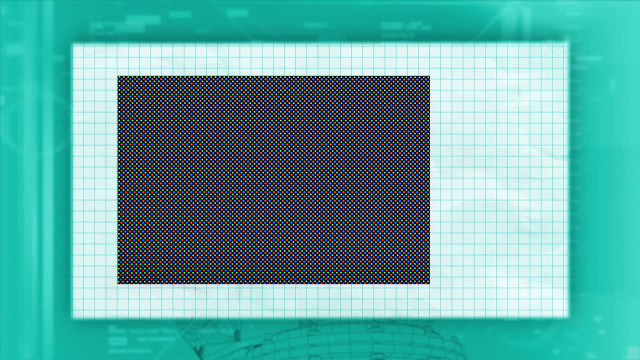 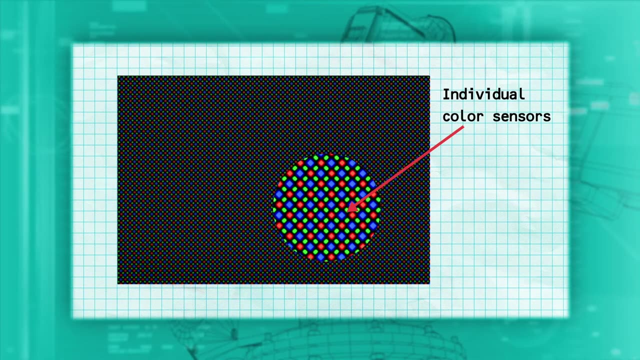 these sensors are measured in millimeters and are about the size of a fingernail, but can be slightly bigger or much smaller. The sensor is made up of a grid of very small, individual color sensors, similar to the cone cells in your eyes. These small sensors are known as pixels, a term 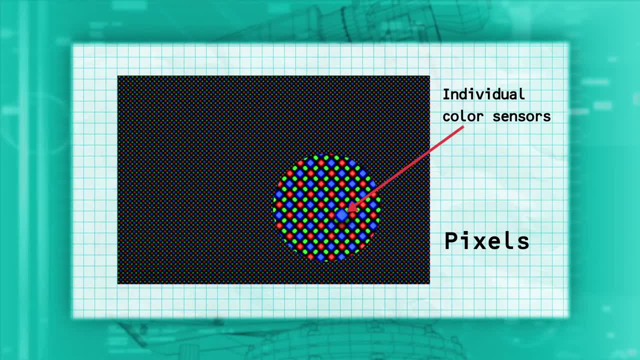 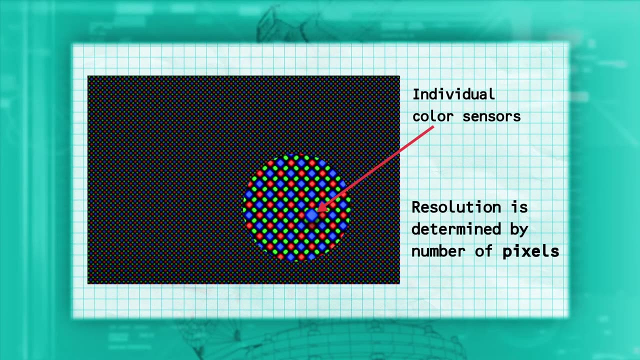 you've probably heard before, Each pixel measures the color of one tiny point in the image. When you put all the small points of color together, you get the full image. The number of these small sensors or pixels determines the resolution of the camera, And for a typical camera there can be. 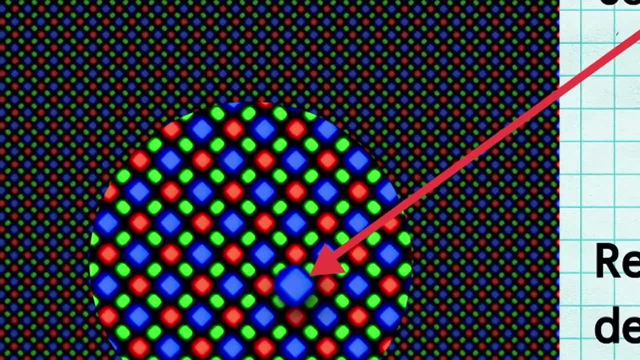 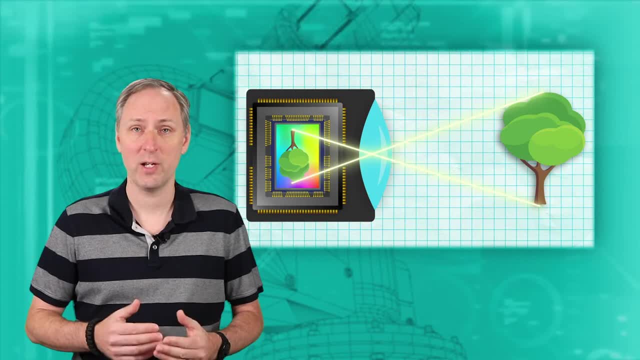 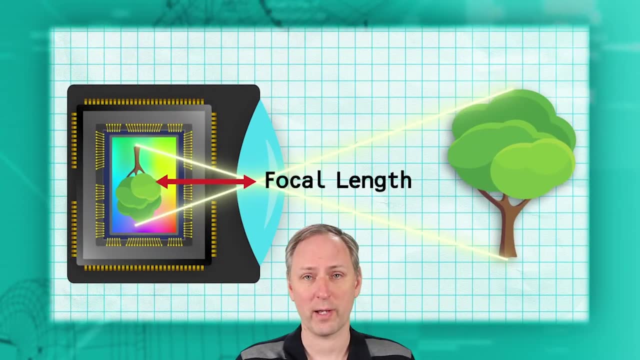 millions of pixels. Besides the resolution and sensor size, the other critical dimension of a camera is how far the image sensor is from the sensor, The lens of the camera. This distance is called the focal length of the camera. We can use the focal length information later to help us determine an object's location. Now let's look at an example. 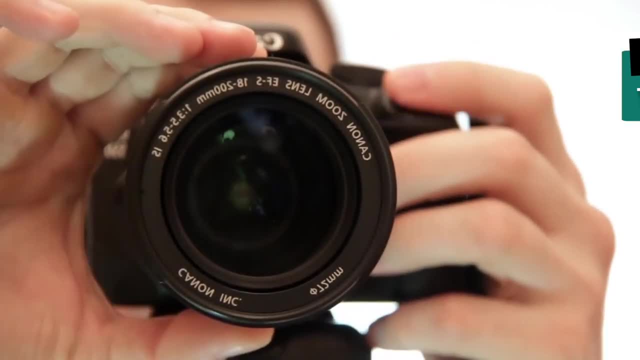 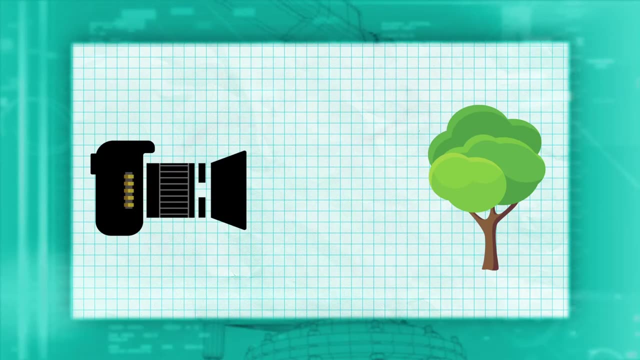 to see how we accomplish our first step: taking a picture. We have our camera and an object, in this case a tree. If we look inside the camera, we can see the sensor and the lens. Imagine the lens as a simple pinhole. 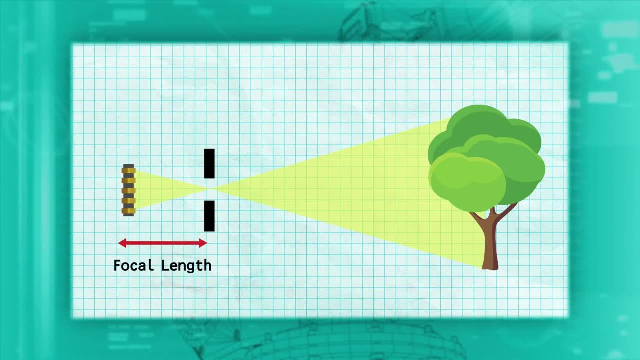 We can see that the image is formed on the sensor at the focal length from the pinhole. We can also think of the pinhole as the camera center. This model of camera is called the pinhole model. We can also see why the tree is upside down on the sensor, since the pinhole takes a ray from the top part of. 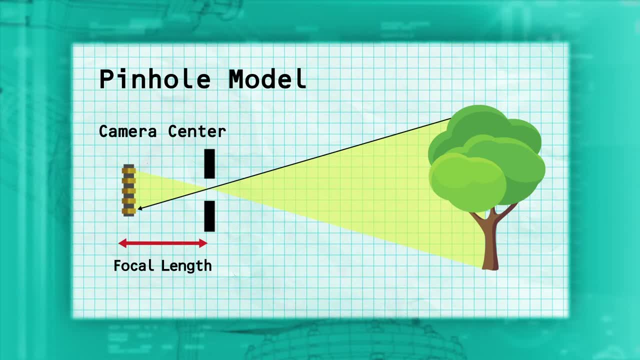 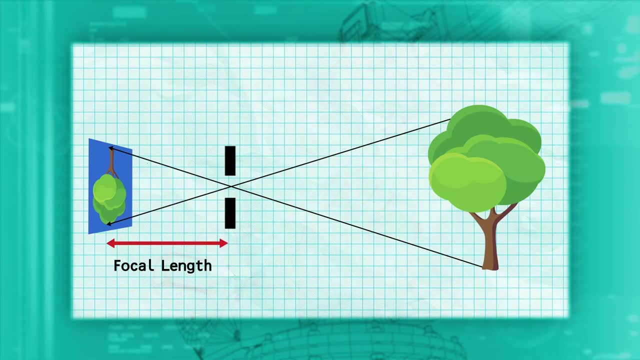 the tree and focuses it on the lower part of the sensor, and vice versa. Dealing with an upside down image isn't very convenient. So what if we were to imagine an image in front of the pinhole? The image would pass through the pinhole at a distance equal to the focal length, instead of behind the hole. 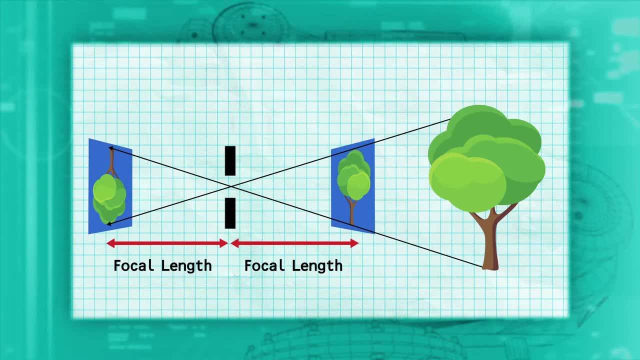 Since the rays from the tree would now pass through the image plane before they went through the pinhole, we would get a right-side up image. We call this new image the image plane, and it's almost always used instead of the actual image on the sensor when describing what the robot sees. 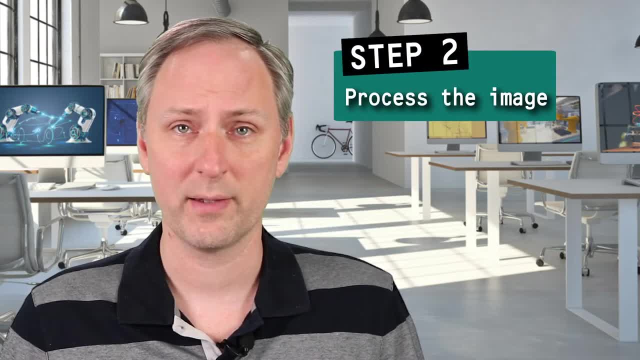 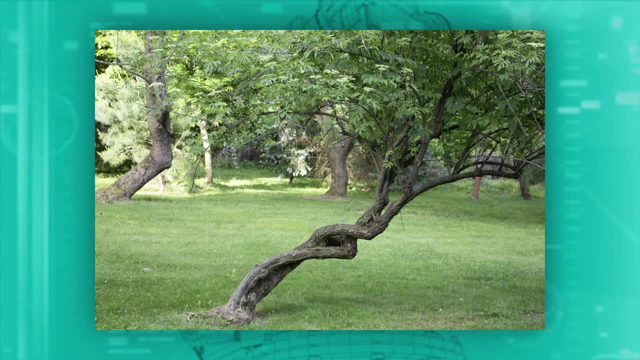 Now that we have our image of the tree, we need to figure out what to do with it. The next step is the image processing step. This step takes a raw image and finds interesting parts. We can find edges or corners of objects, for example. 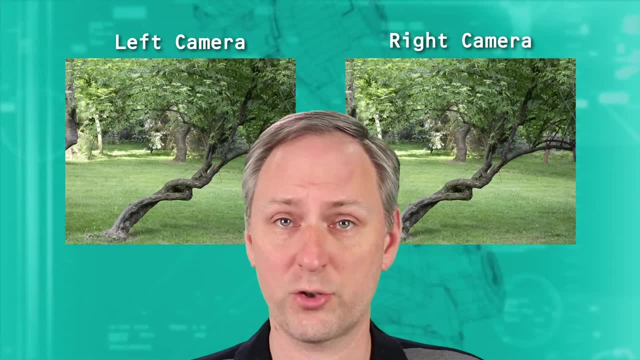 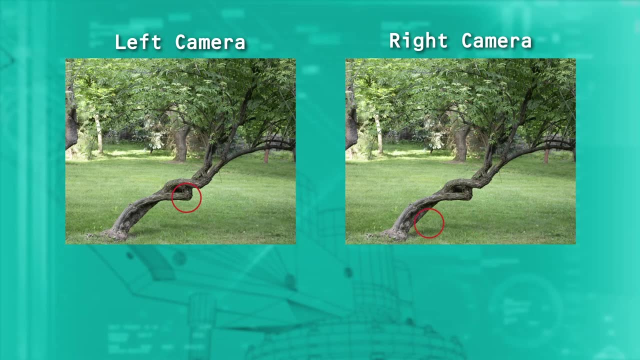 For our example of trying to avoid hitting the tree, we need to find the tree in both images. To do this, we look in both images for some common features of a tree. Features can be anything that the camera system can easily identify, such as unique patterns or corners. 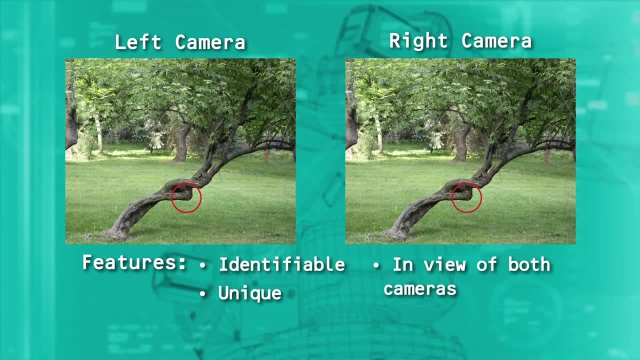 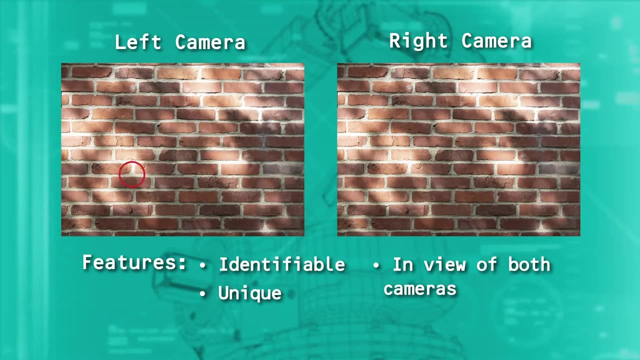 corners. The key idea is that both cameras need to be able to see and identify the features, and they need to be unique. The intersection point of some bricks and a brick wall might be easy to find, but it isn't unique, so you can't. 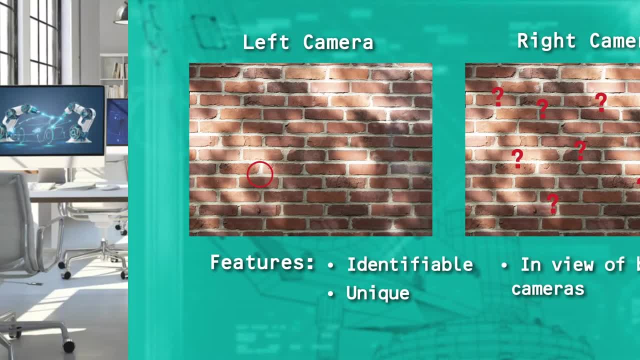 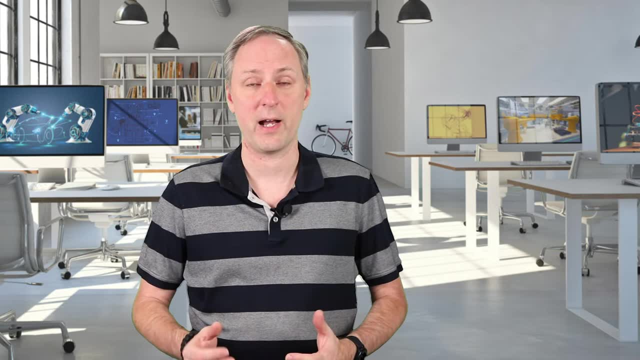 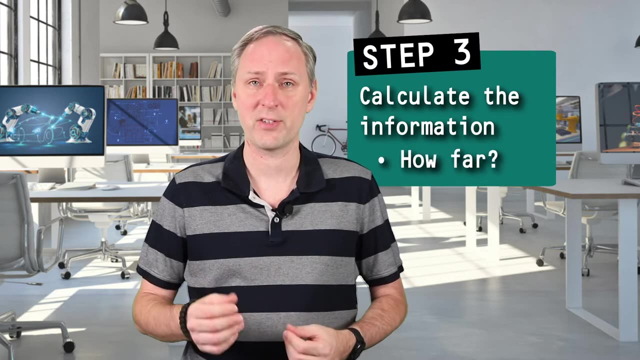 tell which junction you're looking at. The final step is to analyze the images, that is, to calculate information from the features we've identified during the processing stage. One bit of information that the robot often wants to know is how far away are the things I can see from me For our tree avoidance example? 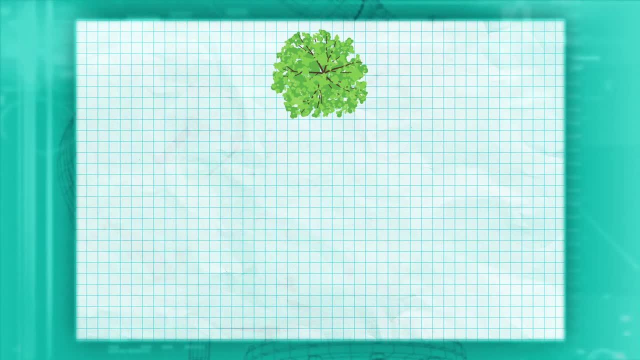 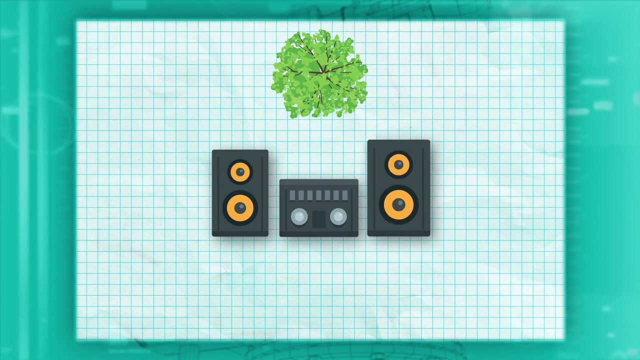 we want to be able to use these features to determine how far away the tree is so we can turn early enough to avoid a collision. One way of doing this is by using a stereo camera setup. Just like stereo sound produces different sound signals for your right and left ear. 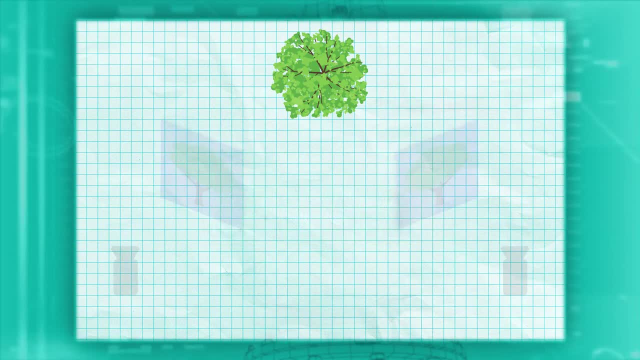 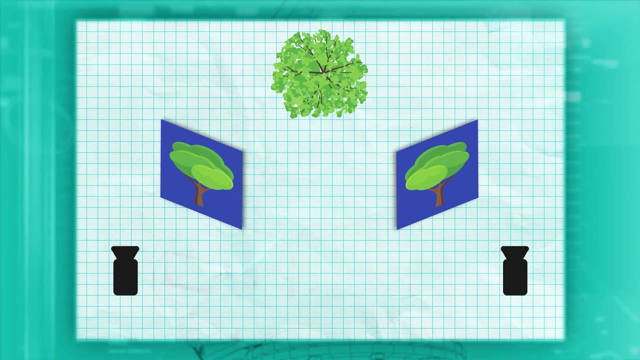 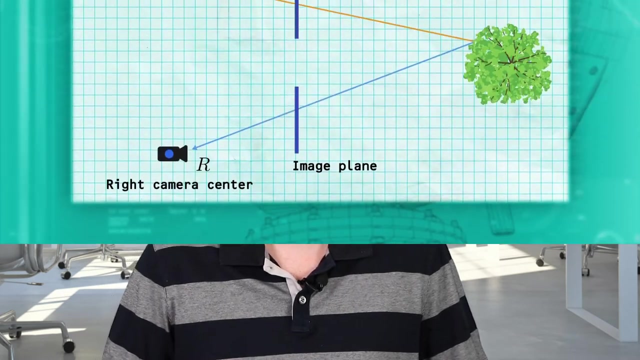 stereo cameras collect two simultaneous images, with a right and left camera. The stereo cameras are arranged parallel to each other and are a known distance. apart From the simultaneous images they collect, we can calculate where the tree is relative to the cameras. Let's start by looking at our setup from overhead. We 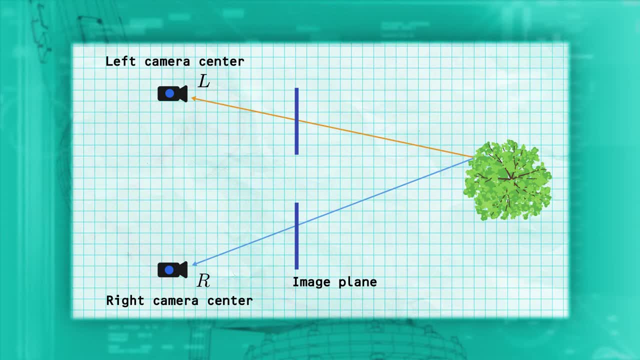 have our tree in front of the robot and two cameras on the robot mounted 50 centimeters apart. If there is a feature on the tree at a point P, then it will appear on the image plane on the left camera at point A and at point B for the 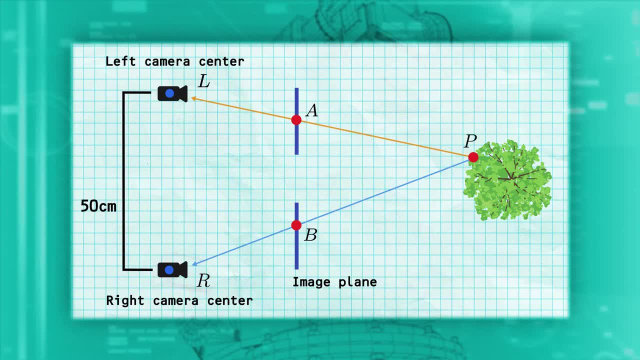 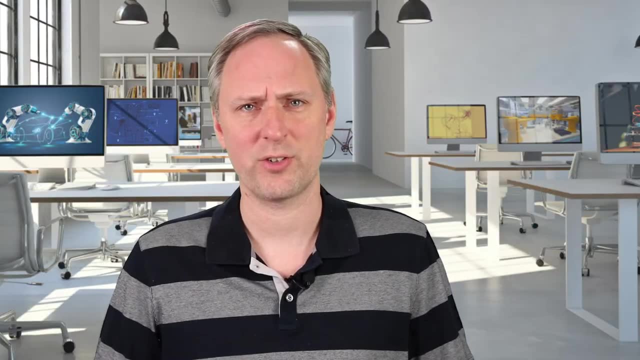 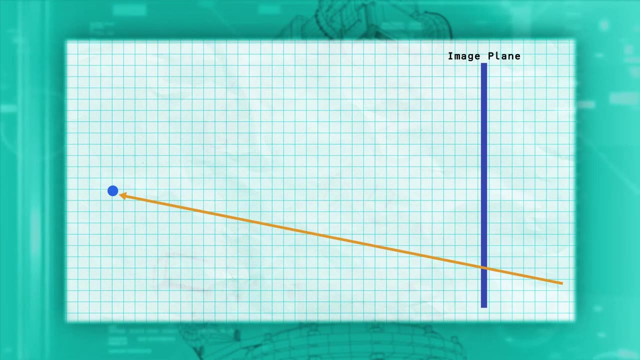 right camera. We also know the camera characteristics: focal length, sensor size and sensor resolution. So how can we determine the distance to the tree from this information? Let's start by looking at the left camera up close. What we want to know is which way that we can get the distance. We want to know the. 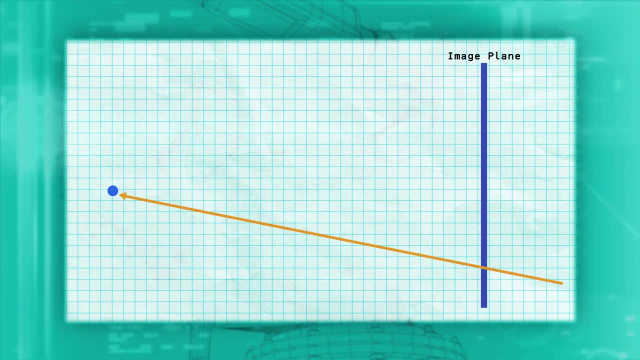 orange ray is pointing. We want the equation for that line. Let's set the left camera center to be at 0, 0, 0.. We know the camera characteristics. in this case, the focal length is 50 millimeters. the sensor is 10 millimeters wide. 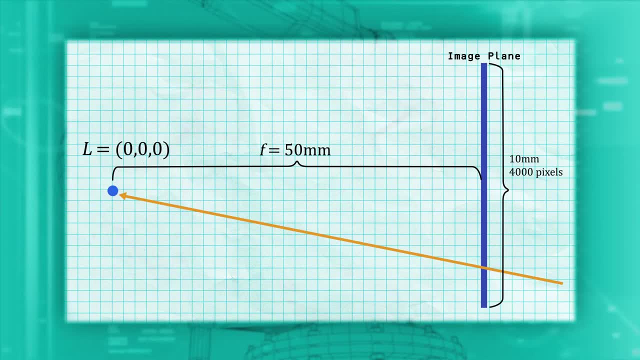 there's also 4,000 pixels wide. We know that the image plane is the XY plane, so the Z axis is perpendicular to that and points out in the same direction the camera is pointing. We also know where our point P shows up in our image. that 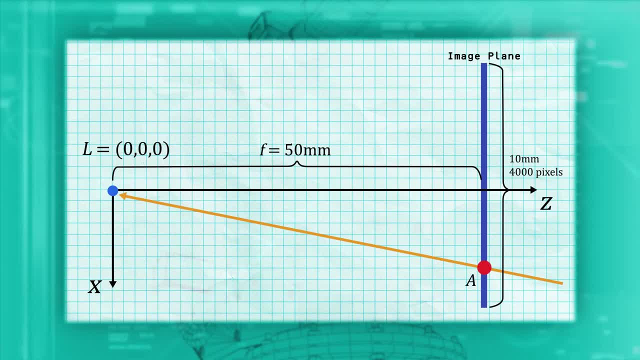 is. we know the X coordinate for point A on the image plane. We know that the Z axis goes to the middle of the image plane at point C, so the X coordinate of C is 0.. We also know that since C is in the middle of the sensor, it is 2,000. 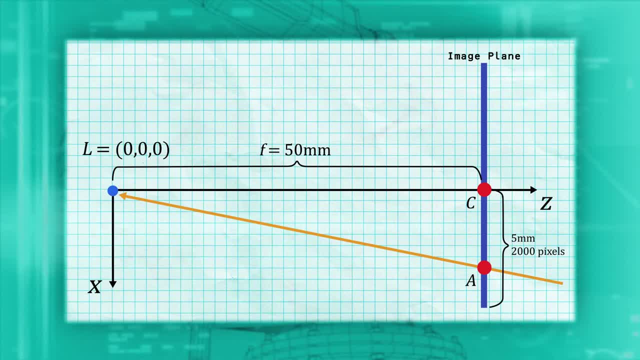 pixels from the right and left edge of the sensor. Let's say the feature we are looking at is at a pixel 2800, meaning the unit is 800 pixels to the right of center. Since the sensor is 10 millimeters wide, it is 5 millimeters from the center to the edge and also 2000. 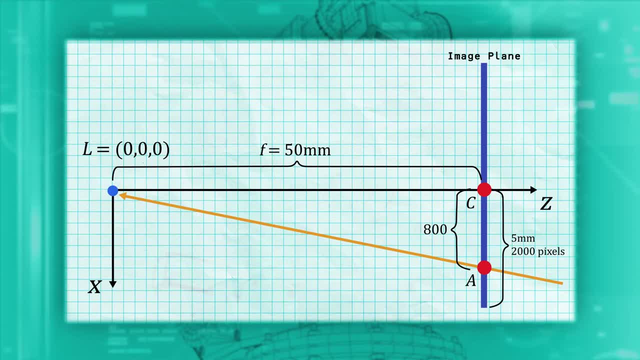 pixels from the center to the edge. Taking our pixel coordinate for point A, we multiply it by our ratio of 5 millimeters per 2000 pixels and get an X position of 2 millimeters. Now we know the location of the point. 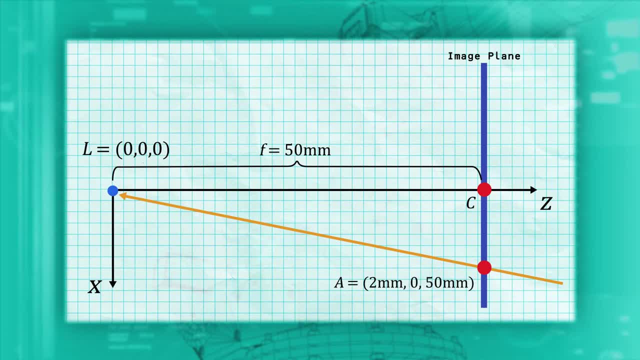 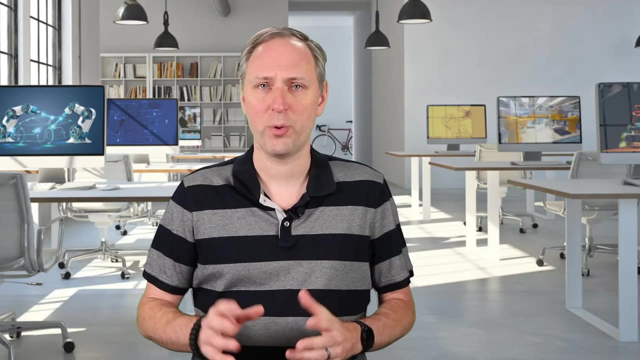 on the image plane corresponding with our feature, X equals 2 millimeters and z equals 50 millimeters. we also know that the line must go through the camera center. x equals 0 and z equals 0.. from this we can create the equation for a line through two points: z minus. 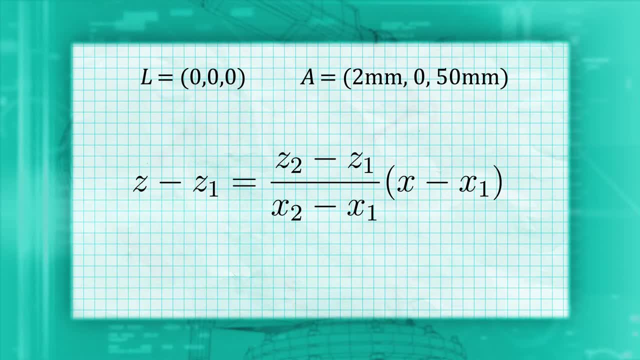 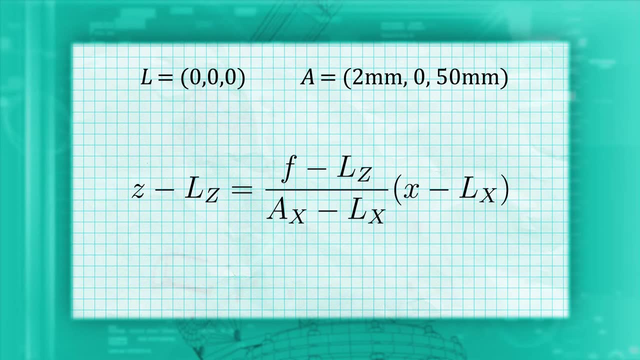 z1 equals z2 minus z1, divided by x2 minus x1, multiplied by x minus x1. we already know some elements of this equation. we will set point two to be the feature on the image plane at point a, which is located at the focal length along the z-axis at the x-coordinate we have already found. 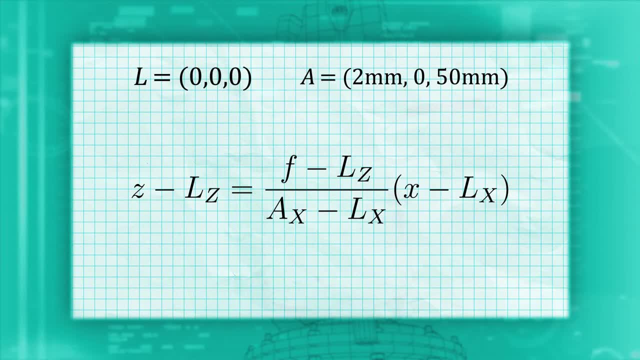 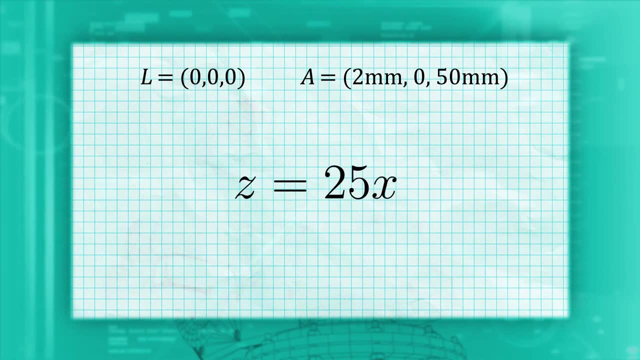 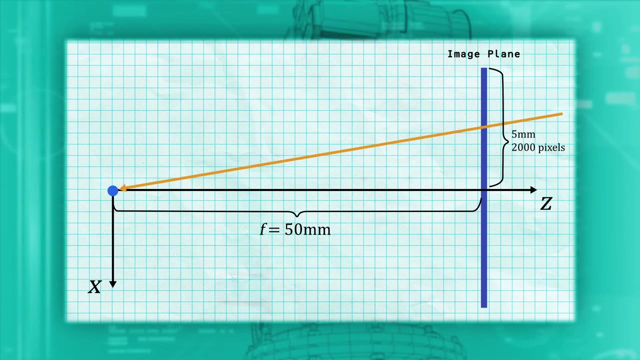 we also know that the point one is the left camera center and is at zero zero. we can simplify and substituting in our values, we see that we get z equals 25x. we can do the same thing for the right camera. in this case, the camera center isn't at zero, zero, zero anymore, since the camera is mounted in a. 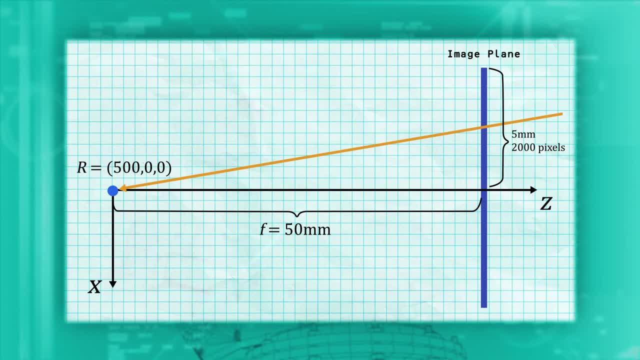 different position. for our example, the cameras are mounted 50 centimeters apart, so the camera center is at x equals 500 millimeters and z equals zero. just as for the left camera, we will start with finding the distance from the sensor center to the point b. in this case, the feature is centered. 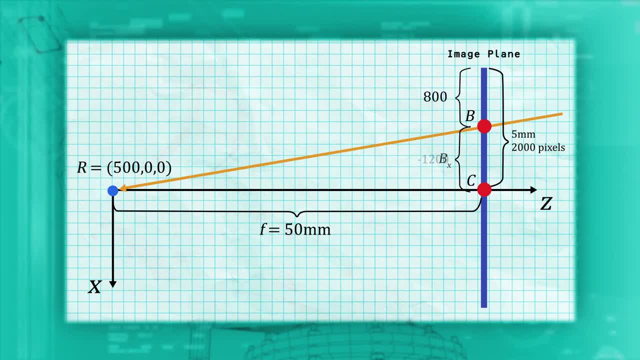 at an x coordinate of 800 pixels or 1200 pixels to the left of center. multiplying negative 1200 by our ratio of five millimeters per two thousand pixels, we get a x position of negative three millimeters. however, remember that the origin is centered at the left camera center, so the true x position is 500 millimeters. 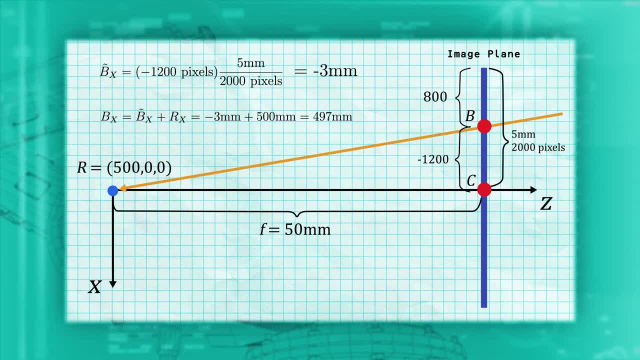 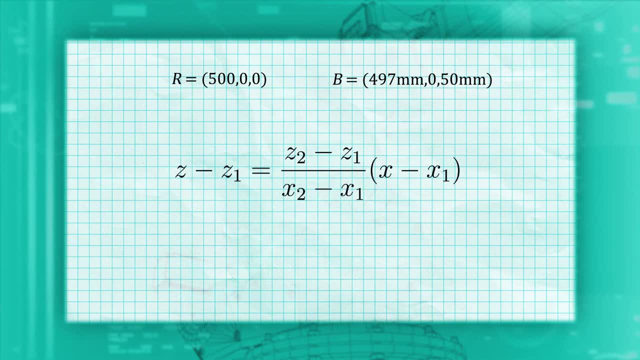 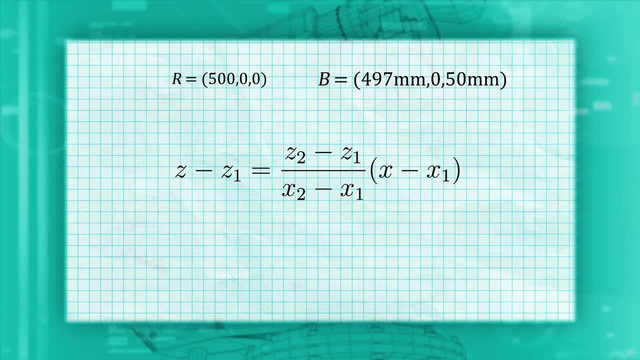 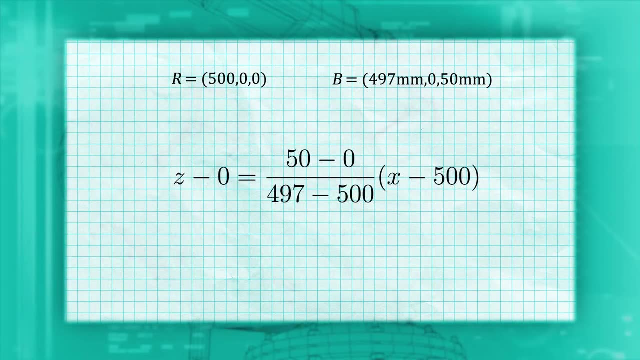 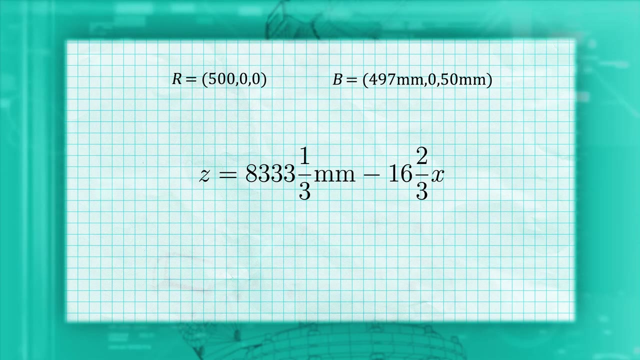 b coordinate and has a z value equal to the focal length and point one is at 500 zero. we substitute in the values and simplify and we get our final equation: z equals 8333 and one-third millimeters minus 16 and two-thirds times x. 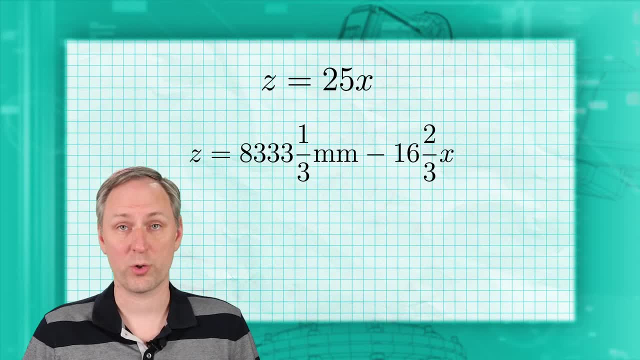 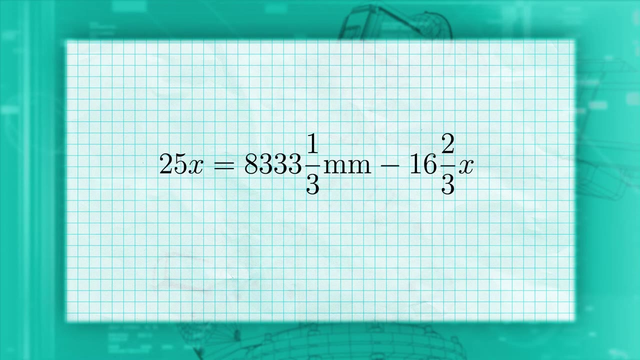 now we have two equations with two unknowns: x and z, the actual position of our point p in the real world. we can solve this system of equations by substitution, since they have z terms with a coefficient of one. we can then rearrange the equation to solve for x and we get a value of 200. 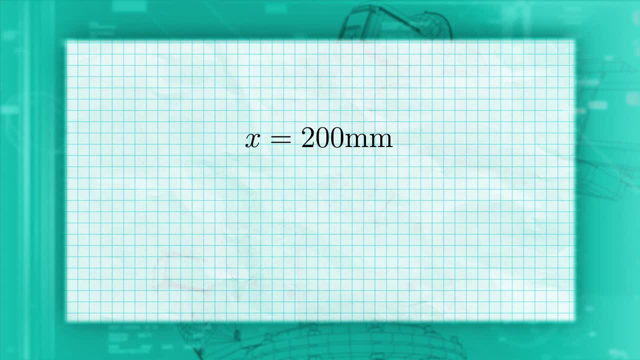 millimeters for x. now substitute that back into either equation and we get our final equation of two hundred millimeters for x. to find the z value in this case we'll use the equation for the left camera and we find that the z coordinate is five thousand millimeters or five meters, which is about 16 feet. 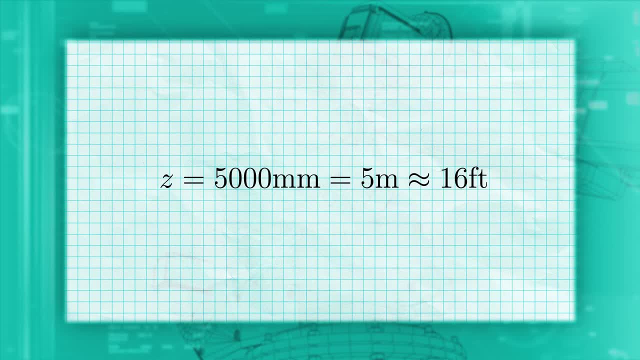 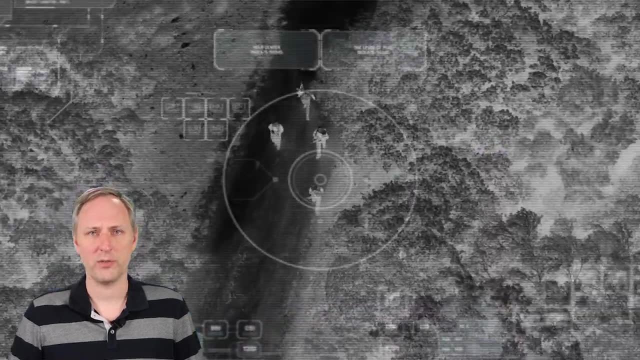 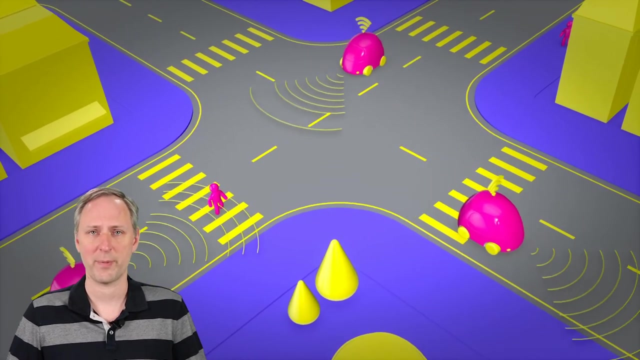 and that is our answer. the tree is at five meters in front of our robot. with these skills, the robot can now put its vision system to good use: identifying the objects around it, interpreting signs in the environment and avoiding obstacles, all with a single type of sensor. now get your pencils ready for this week's challenge questions. 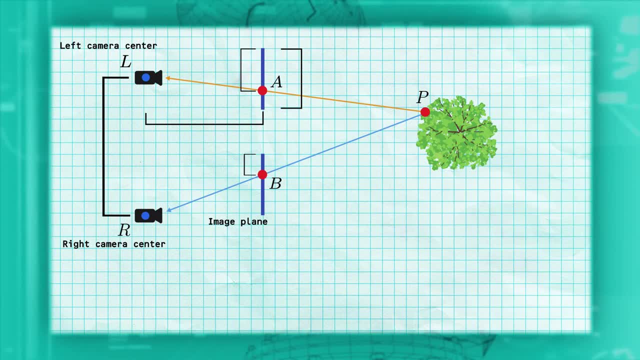 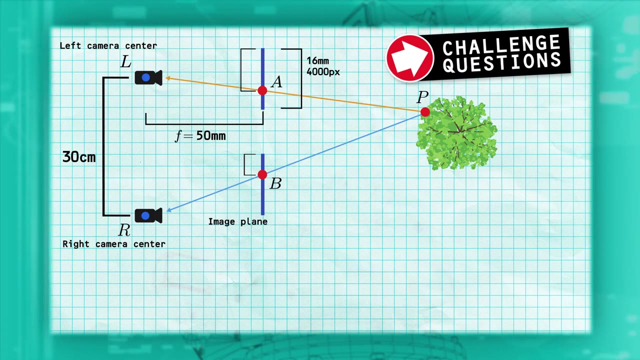 a robot with the stereo camera pair mounted 30 centimeters apart, with a 50 millimeter focal length and a sensor that is 16 millimeters wide with 4 000 horizontal pixels. question one is if a feature on an object is located: an x coordinate of 3 000 on the left camera and an x coordinate of 1 000 on the left camera and an x coordinate of 1 000 on the left camera will the alternate function? if the lines are located 3, 0 on the left and 1, 0 on the left hand side of the object, this will be the linear random dimension of the object and that will be the lane will be crossed at the end of the 19th and 20th ع Waltz will have the objective of a perfect line with a tails and a wt all over. the object will be the linear on the other side line with a left and a y coordinate oforal on the left angle so that the箴 will be: 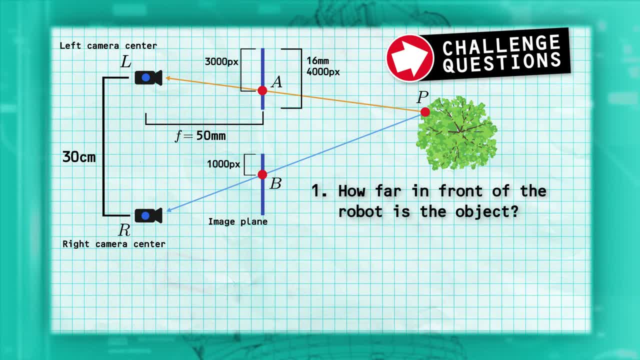 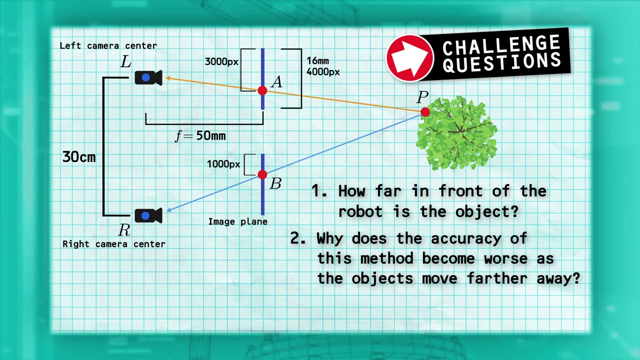 1000 on the right camera. how far in front of the robot is the object? Again, that is 3000 on the left camera and 1000 on the right camera. Where is the object? Question two is: why does the accuracy of this method become worse as the objects move farther? 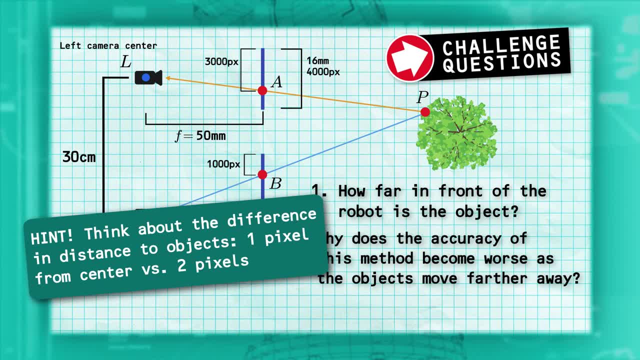 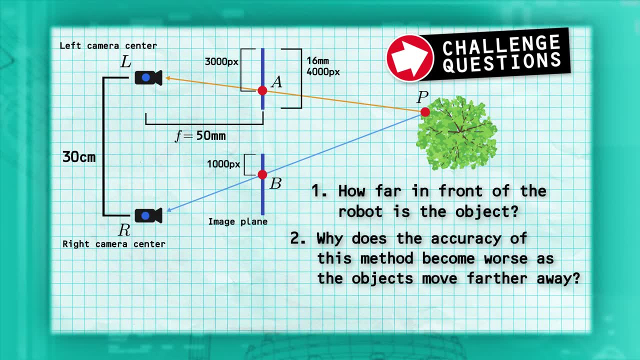 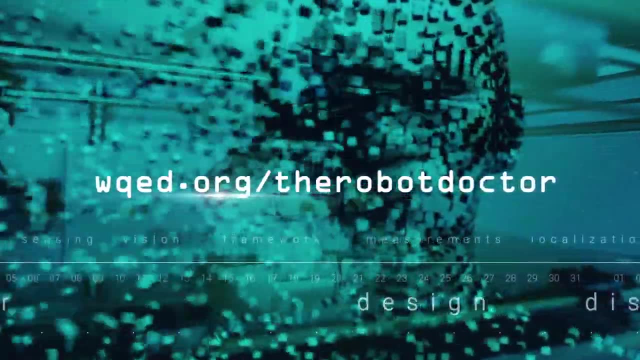 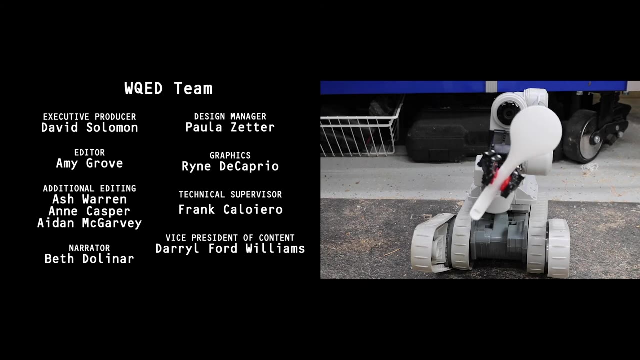 away. It may help to think about what the distance is if the objects are one pixel from the center versus two pixels from the center. I'm John the Robot Doctor. See you next time. You can find these video lessons at wqedorg: slash the robot doctor. Hey robot, what are you doing? you.